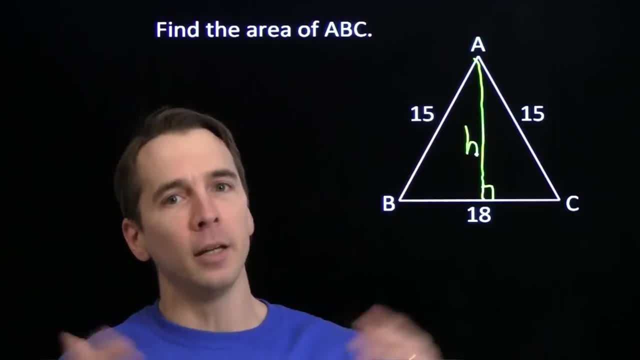 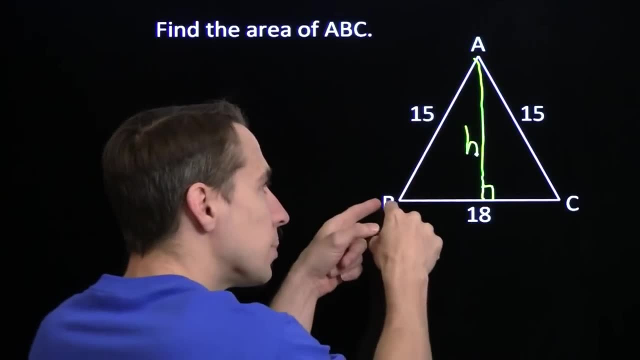 enough. in law or politics You lay a little bit of probably out there and you can convince people, But in math probably isn't good enough. We're going to prove that when we draw this altitude, we split the base down here into two equal lengths, And the way we'll do that. 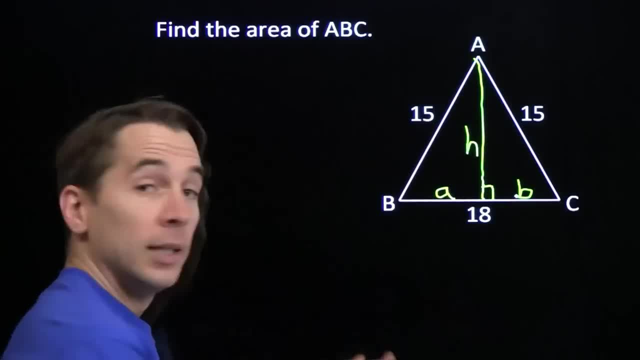 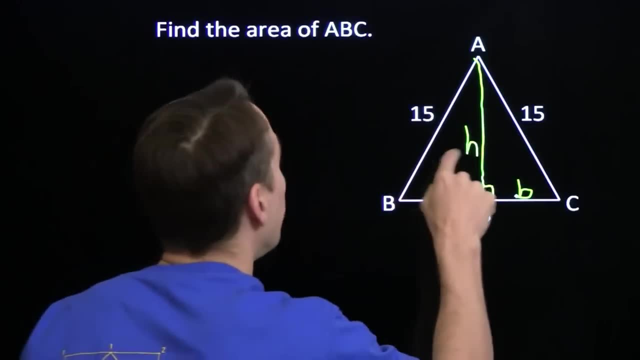 well, we'll start off. we don't know what they are, We'll call them a and b. Now we have two right triangles. We have two right triangles here, so we can apply the Pythagorean theorem to both of them. 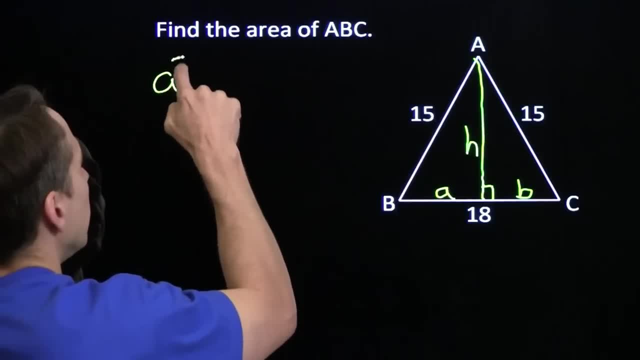 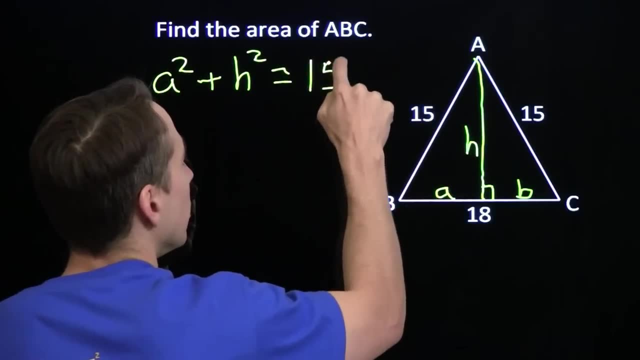 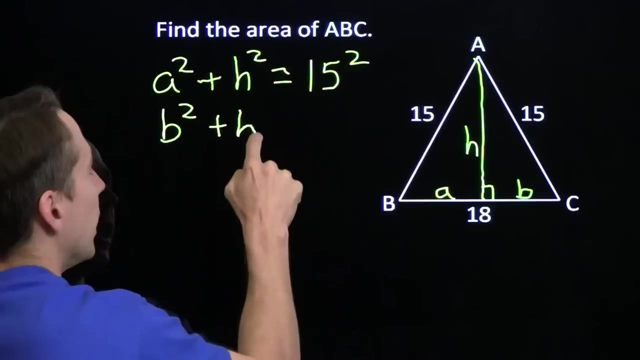 So for this one, the sum of the squares of the legs is a squared plus h squared, and that has to equal the square of the hypotenuse here, 15 squared. And then we have this right triangle. Play the same game over there: b squared sum of the squares of the legs plus 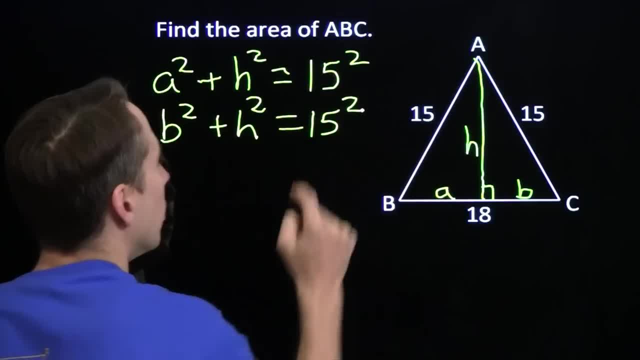 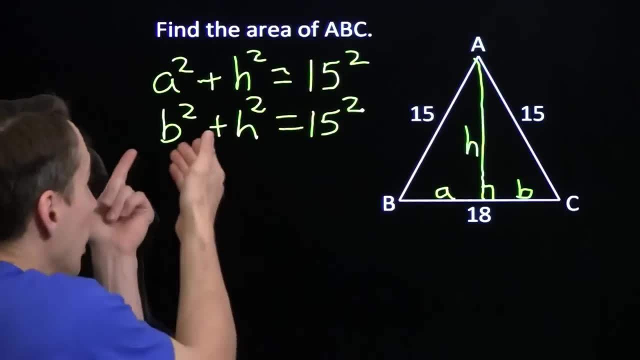 h squared equals 15 squared. And now we can see from these two equations: a squared, that's what we add to h squared to get 15 squared. b squared is also what we add to h squared to get 15 squared. If 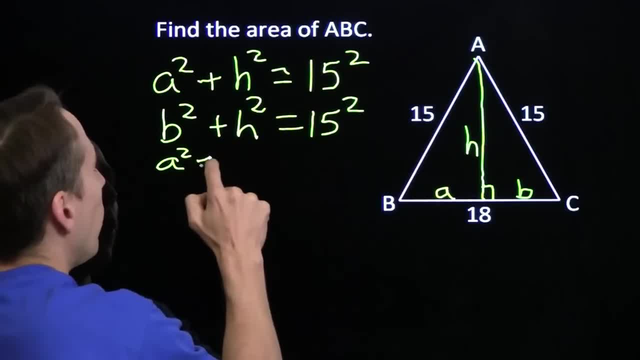 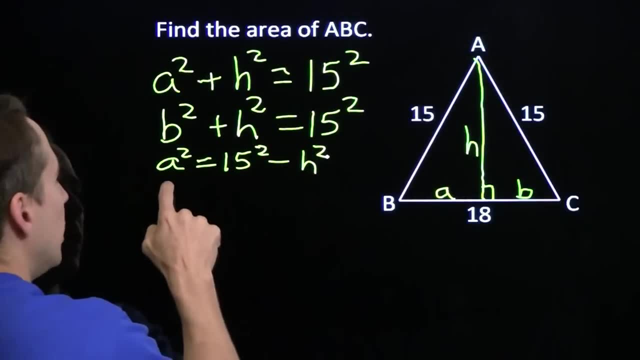 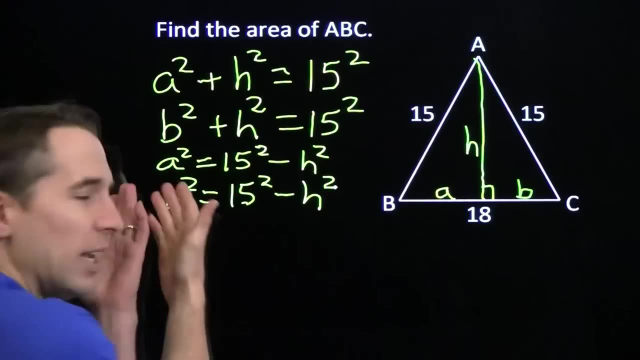 you're not convinced, we can subtract h squared from both sides. We've got 15 squared minus h squared equals a squared. Subtract h squared from both sides of this one, We get the same thing. So a squared and b squared have to be equal And of course they're both positive. So 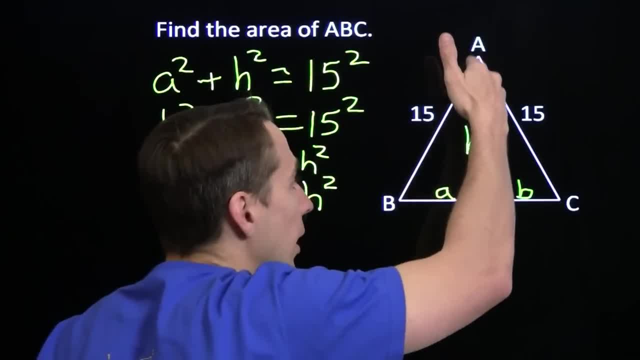 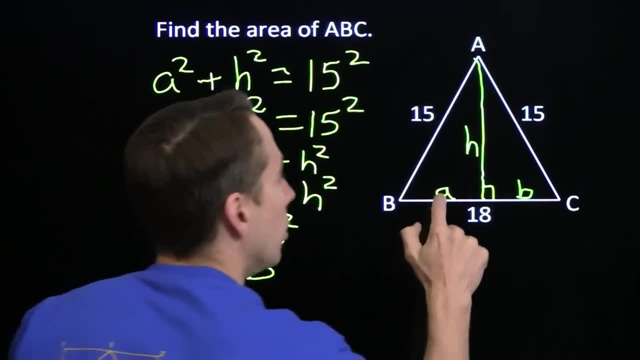 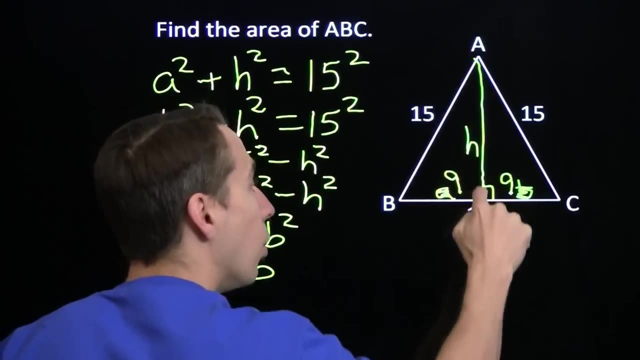 we have a equals b, And that's why, when you draw the altitude here, it splits the base into two equal sides, because these two sides of the triangle are equal. So now we can replace a and b with 9.. And now we have a right triangle, We have one leg, We have the hypotenuse, We can figure. 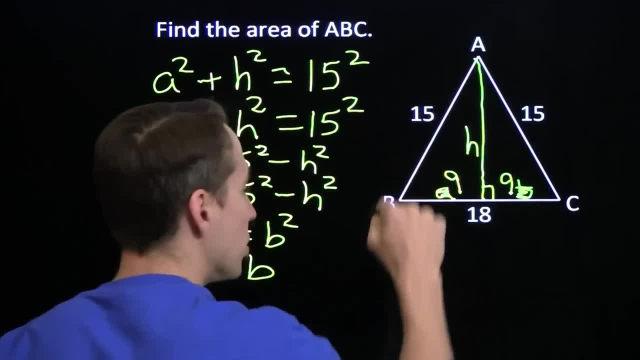 out what h is And maybe you recognize the 3,, 4, 5 right triangle there. But if you don't, you can still just write down the Pythagorean theorem: Subtract: a squared sum of the squares of the legs plus h squared plus a squared. 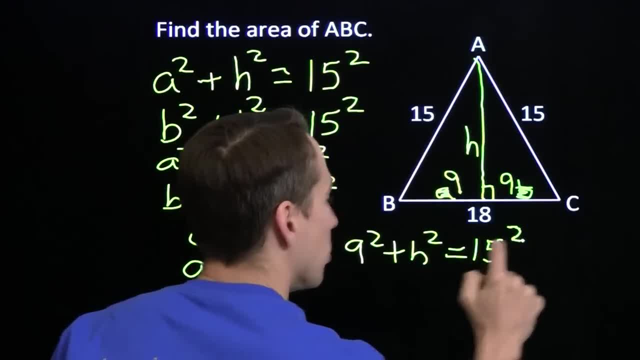 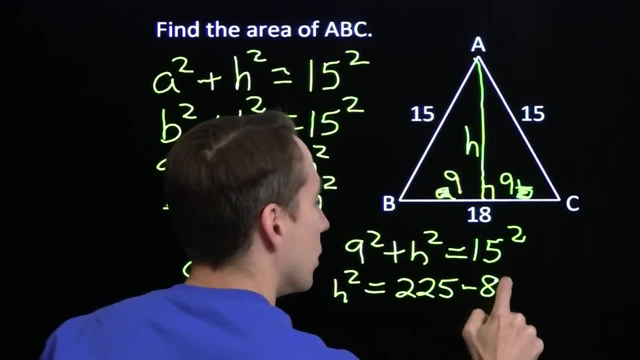 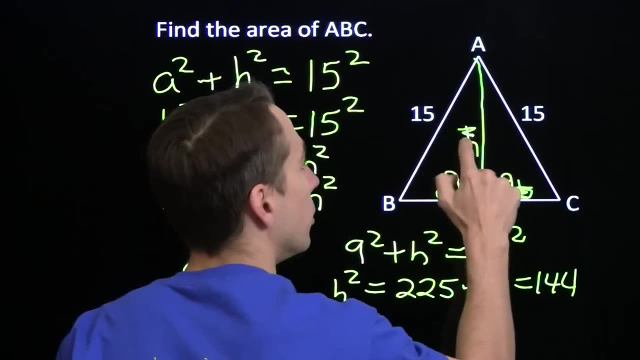 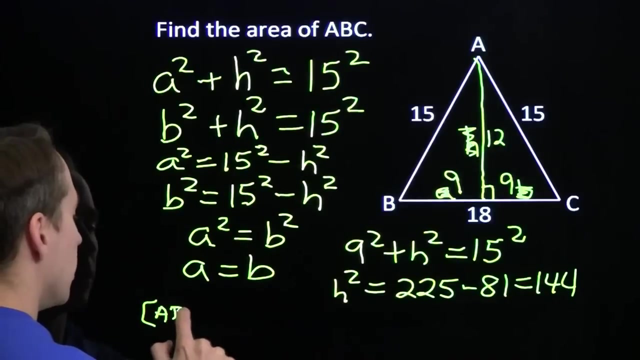 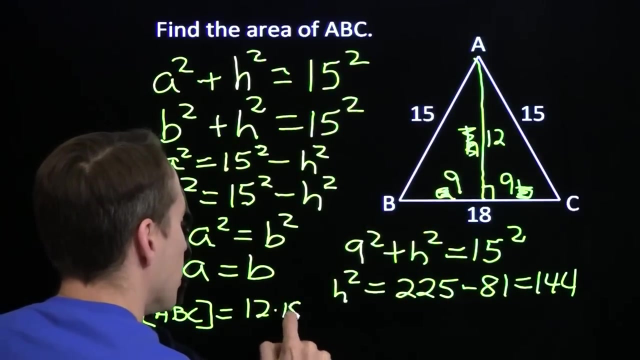 theorem. So you have: h squared equals 15 squared minus 9 squared, which is 144.. So take the square root, we get: h is 12.. And now we can find the area of ABC. The area of ABC is one half. The base is 18.. The height is 12.. 12 times 18 over 2.. Divide the 2 into the 18,. 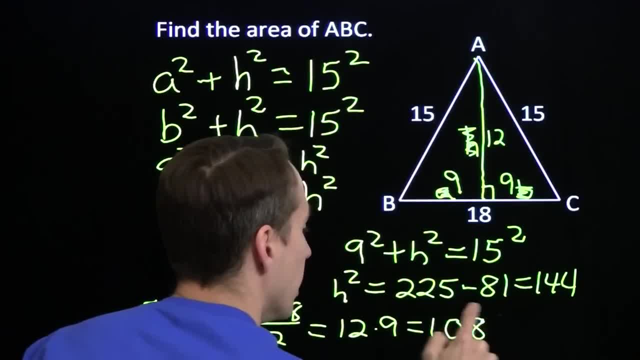 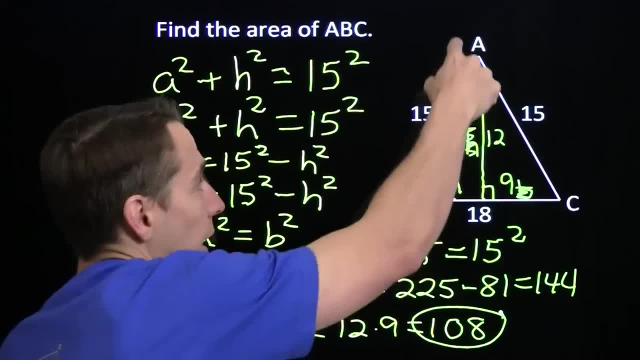 you get 9.. 12 times 9 is 108. And we're finished with this problem. Now, this is a very special triangle. This is called an isosceles triangle- That's what we call it- when two of the sides 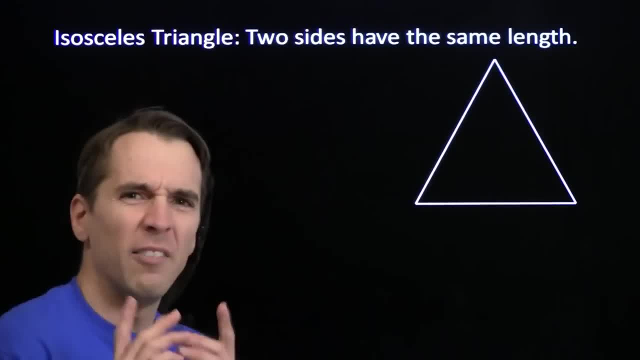 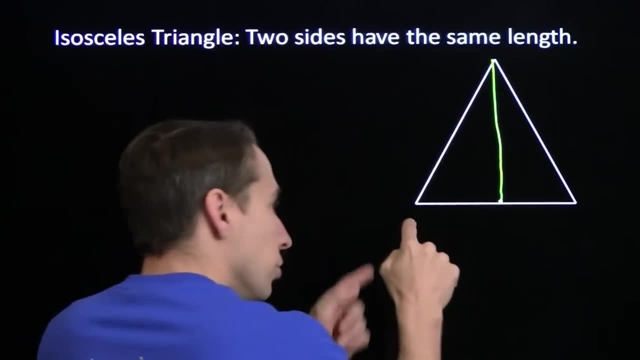 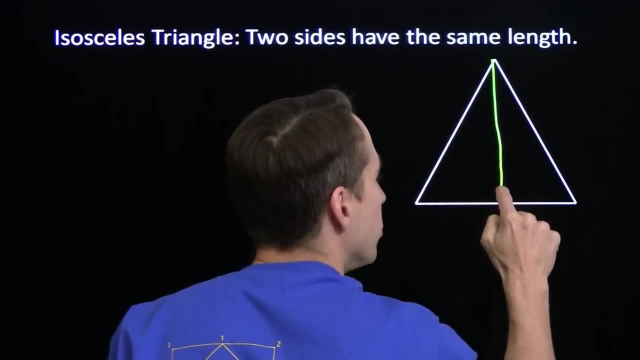 are equal And we saw a very key strategy for dealing with isosceles triangles. When you draw the altitude to the base, the two equal sides are called legs. The side that's not equal to these other two, we call that the base. When we draw the altitude to, 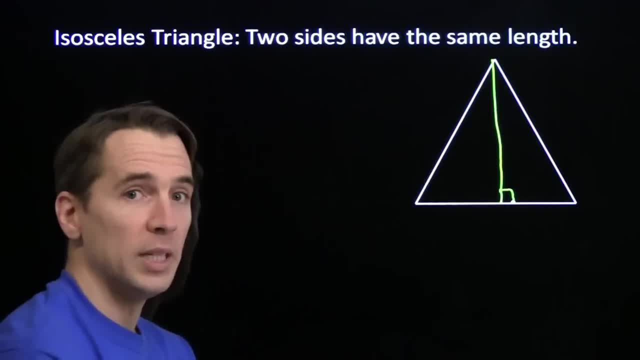 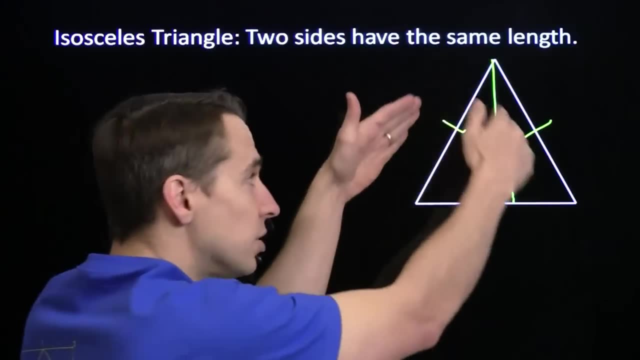 the base. we split the base into two equal pieces. Now one way we show that these two legs are equal is we'll put little tick marks on the sides. These two little tick marks say: these two sides are equal. We've drawn this altitude. It splits the base into two. 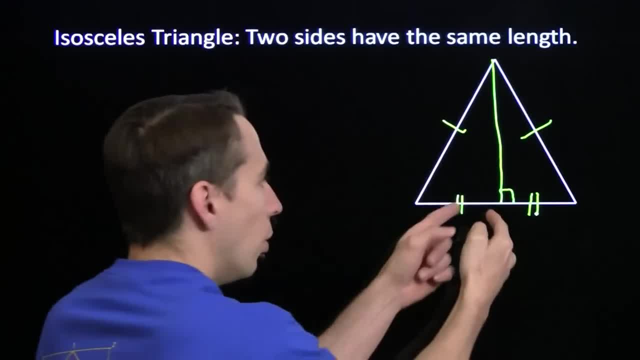 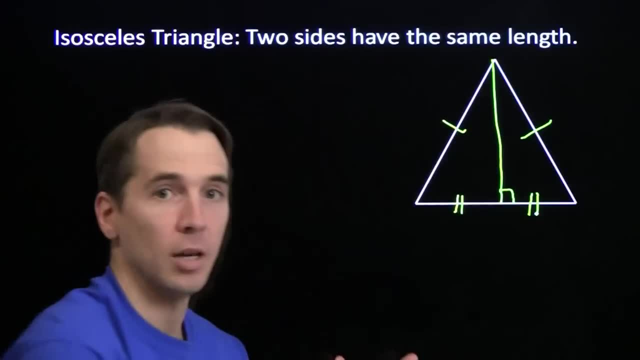 equal sides. We'll put a pair of tick marks on each of these little pieces That says this piece is equal to this piece, but it's not necessarily the same as these two pieces up here Now. this, of course, is obviously the same in both of these right triangles. 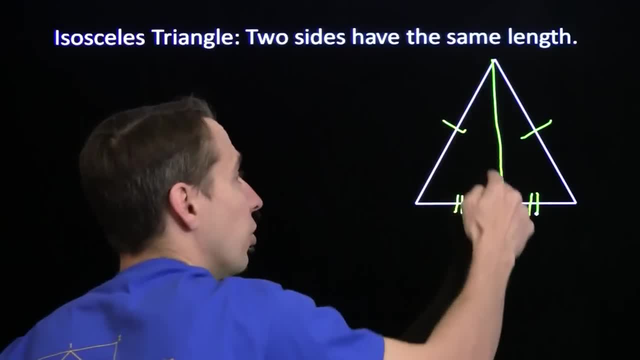 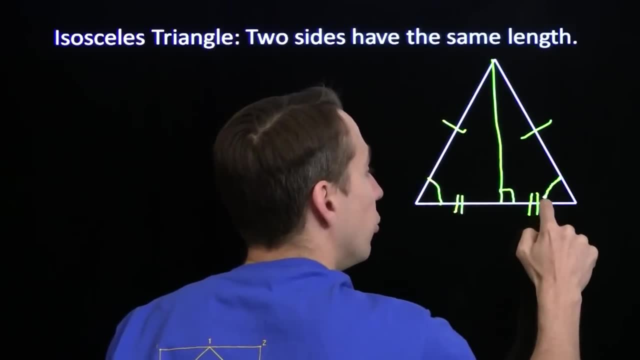 We have a right triangle over here, right triangle over here. The side lengths are the same in each. These two right triangles are identical, So these two angles are equal. So when I look at an isosceles triangle, this is what I see. I see the two equal sides here. 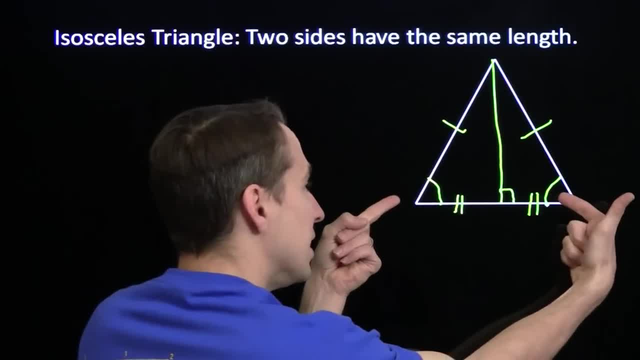 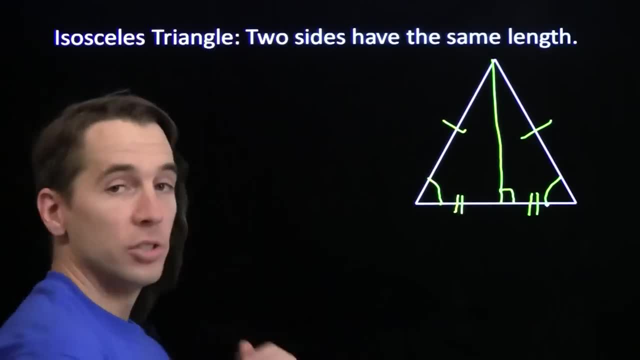 I see an altitude splitting the base into two equal pieces And I see these two. we call these base angles down here. These two are equal. That's the way I think about an isosceles triangle. This also shows us a very key strategy in dealing. 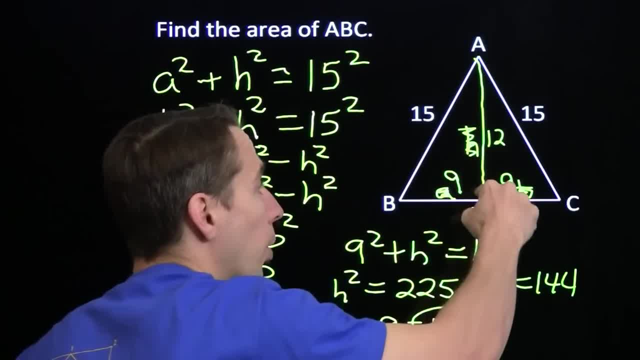 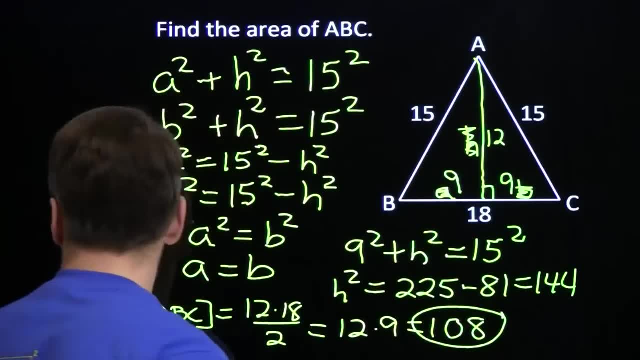 with problems in which we need to find a length, and that is, draw a perpendicular line. Draw a line from somewhere perpendicular to something else. build a right triangle, apply the Pythagorean theorem. Now, there's a very special kind of isosceles triangle, and that's one in which 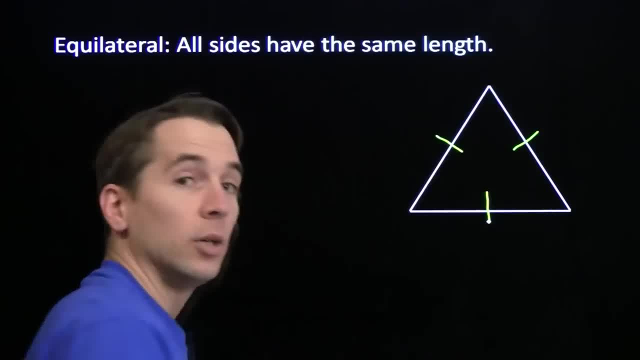 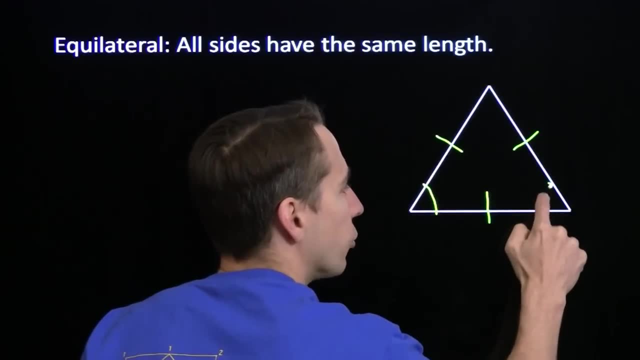 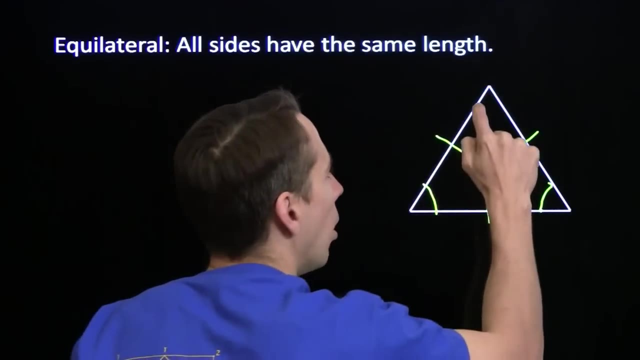 all three sides are equal. We call this an equilateral triangle. Now, of course, because these two sides are equal, these two angles are equal. And well, because these two sides are equal, this angle and this angle are equal. So all three angles have to be the same. Now of, 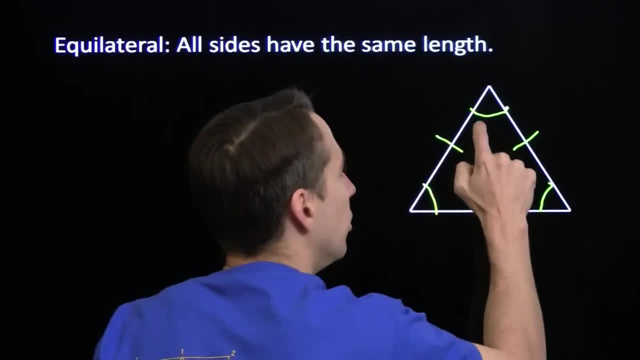 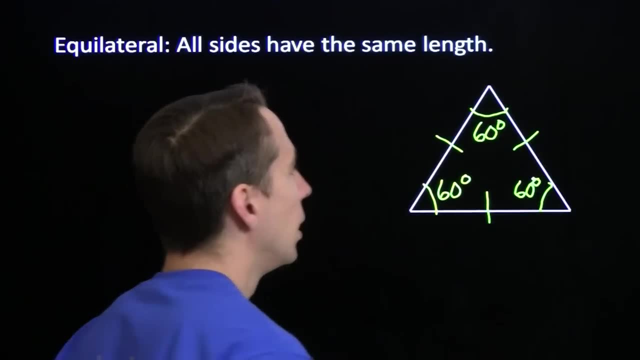 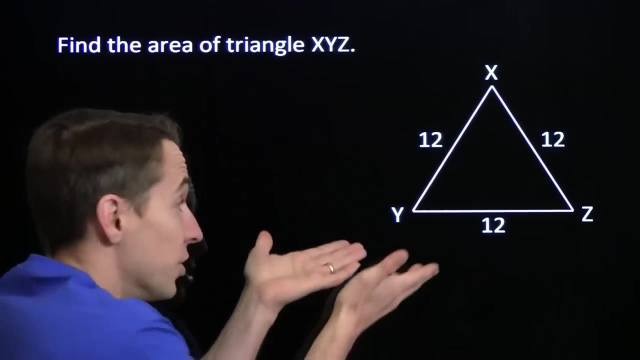 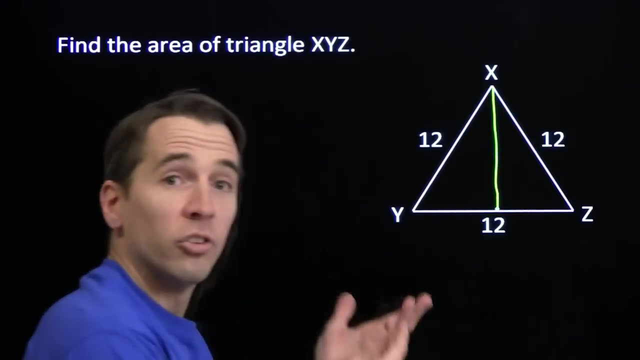 course, all three angles have to add up to 180 degrees, so each of these angles has to be 60 degrees, And we'll finish up by finding the area of one of these equilateral triangles. Now, as equilateral triangles also isosceles, we know what we're going to do here is split. 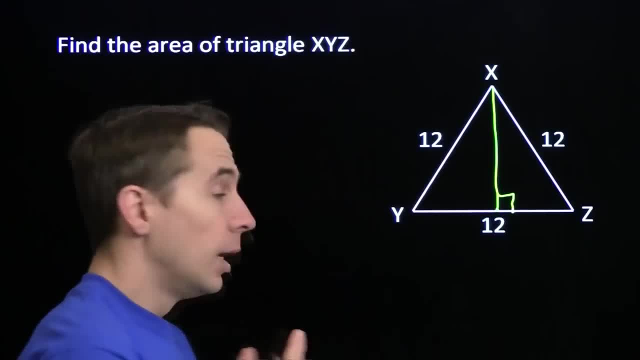 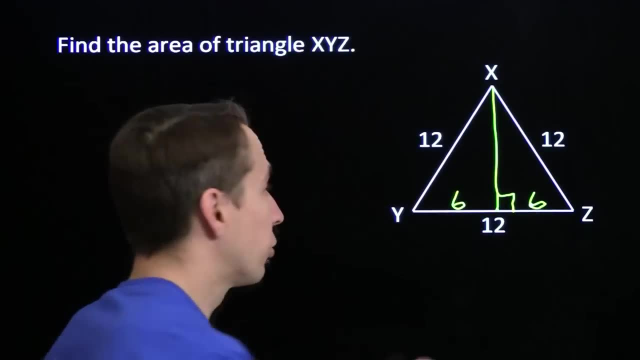 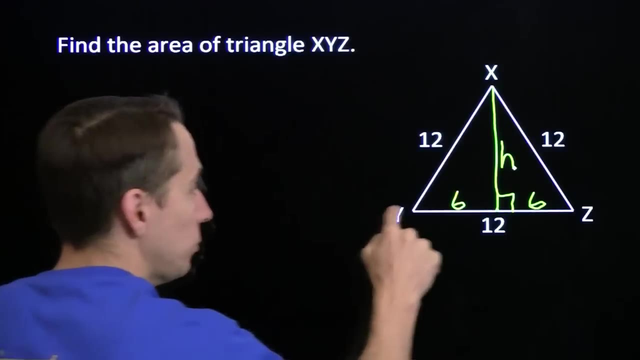 it in half by drawing an altitude. And, just as before, we know that this splits the base into two equal pieces. These each have length 6. And we need to find this height, this altitude, here, So we can find the area. And now we can apply the Pythagorean Theorem. We've got the sum. 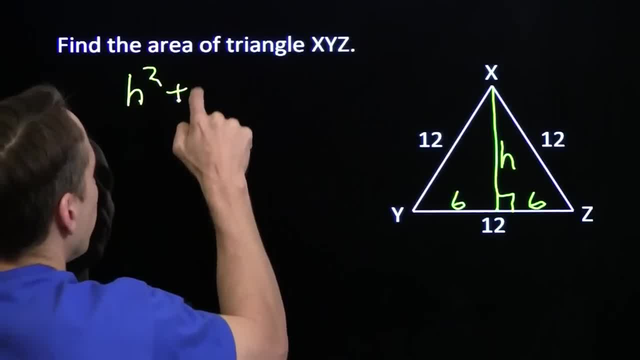 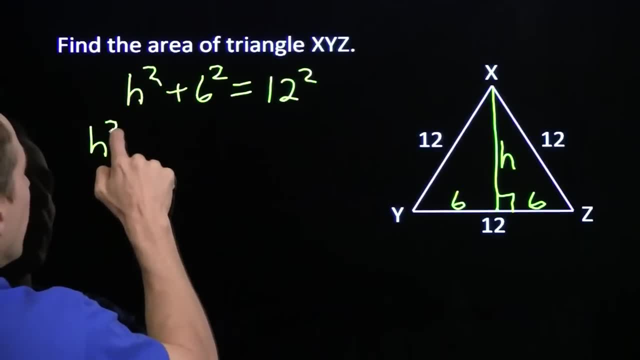 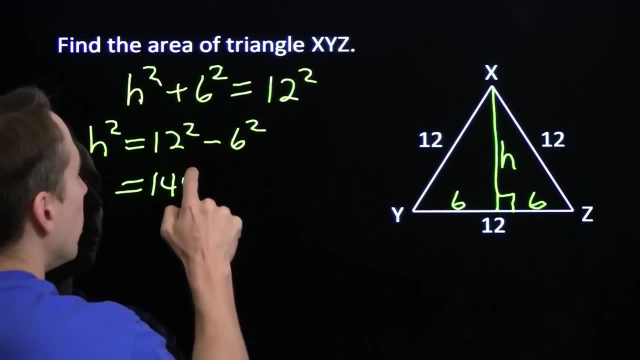 of the squares of the legs. h squared plus 6 squared equals the square of the hypotenuse 12 squared. So we have h squared equals 12 squared minus 6 squared, which is 144 minus 36,, which is 108.. 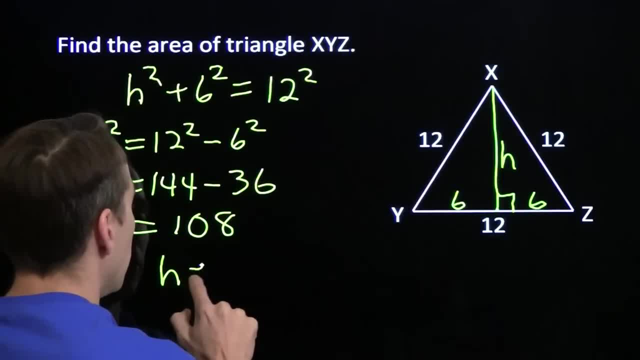 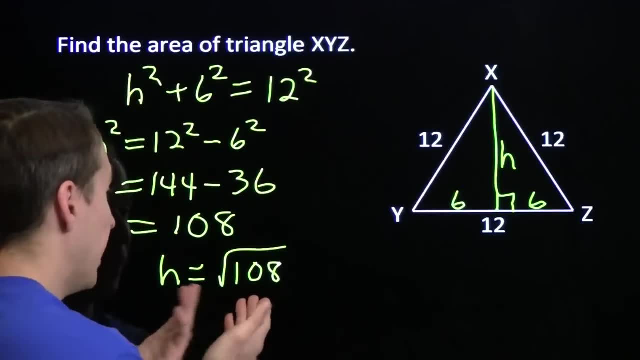 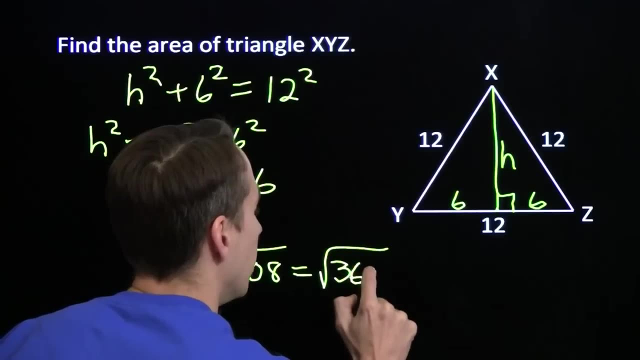 And then to find h, we take the square root of h. Let's take the square root of 108.. We can pull out a factor of 9.. We can also pull out a factor of 4.. This is 36 times 3.. So this is the square root of 36 times 3, which is